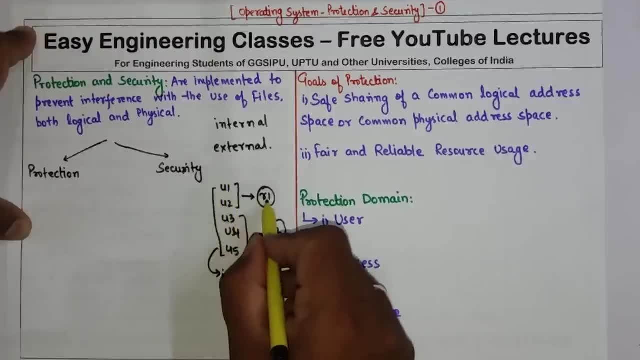 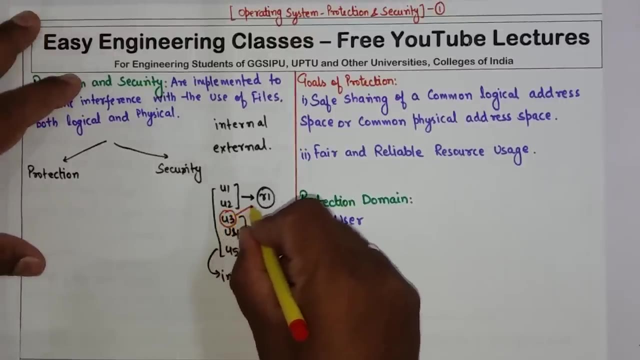 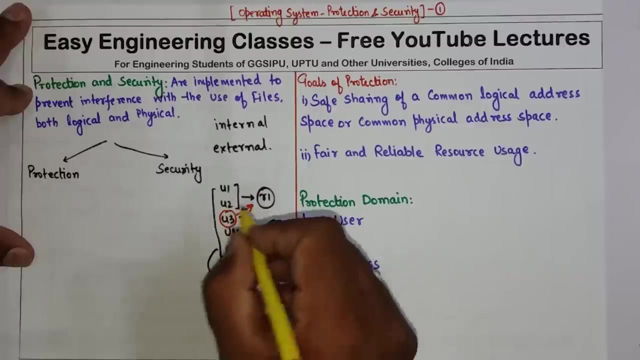 So in this manner these two users can only access resource r1 and these three users can only access resource r2.. But suppose if the user u3 tries to access the resource r1. Then that comes under the protection technique, Because we have to implement certain access mechanism so that a legal or legitimate users can only access a particular resource. 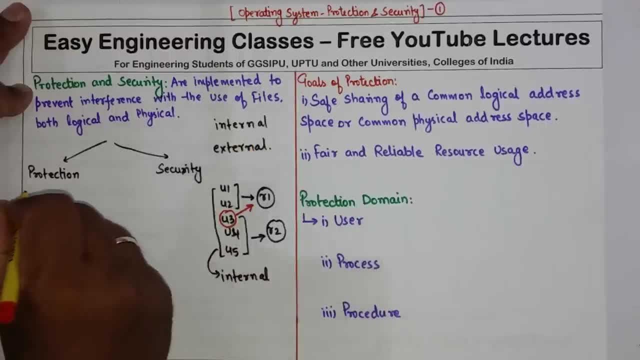 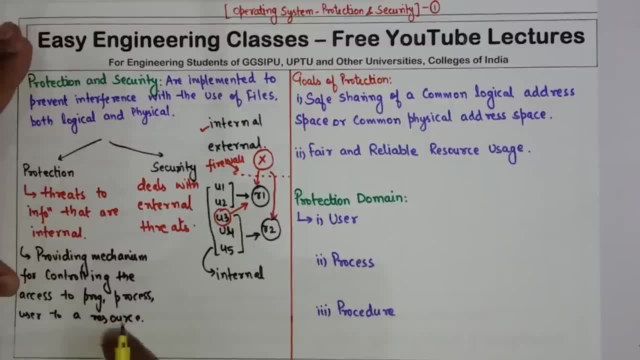 So it is used to deal with the threats to information that are internal threats. So it is used to deal with the threats to information that are internal threats. So it is used to deal with the threats to information that are internal threats. So access to a resource is controlled with the help of protection mechanism. 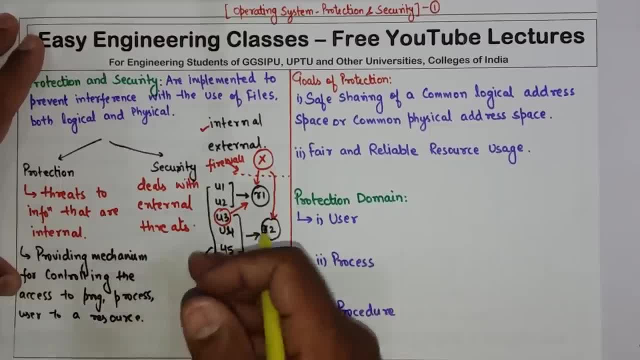 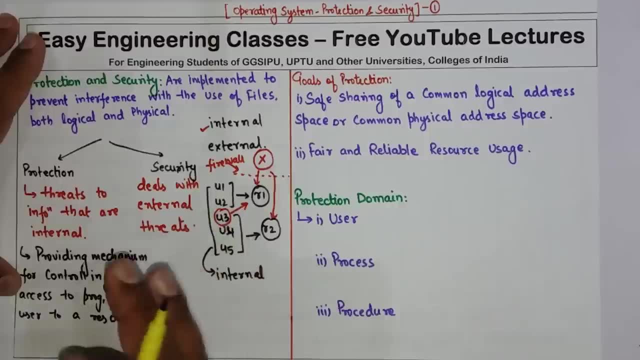 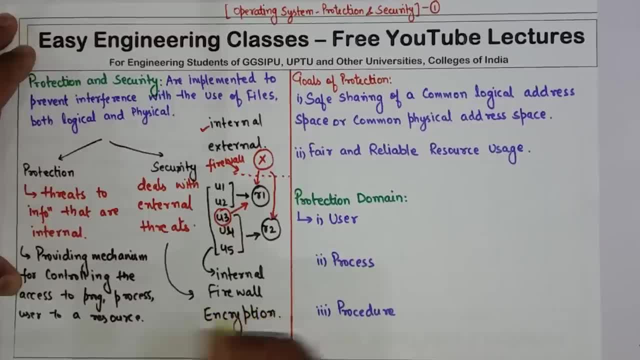 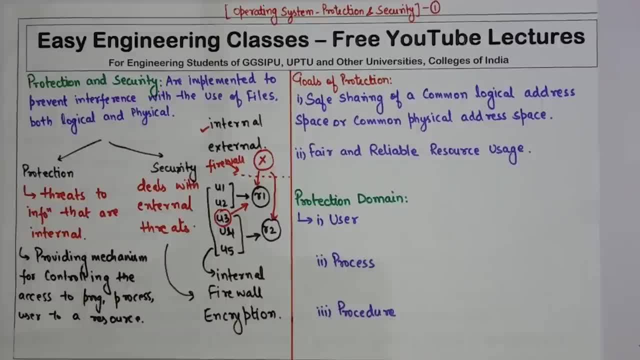 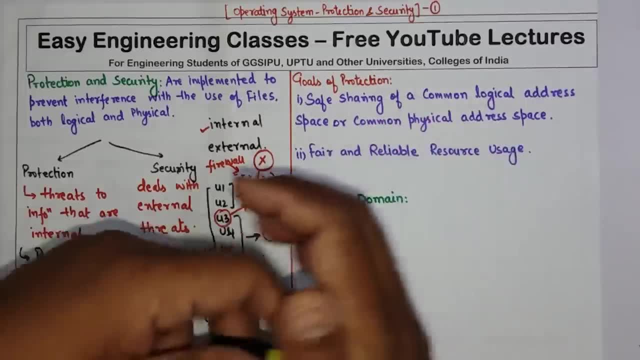 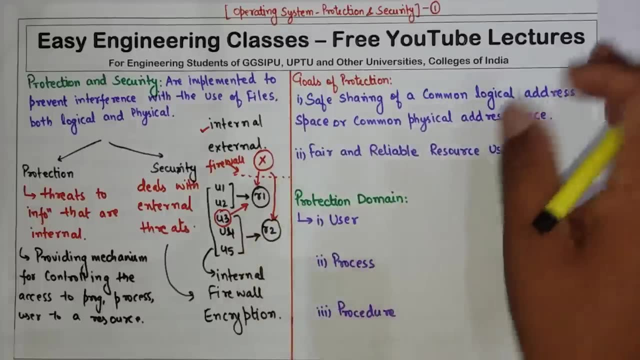 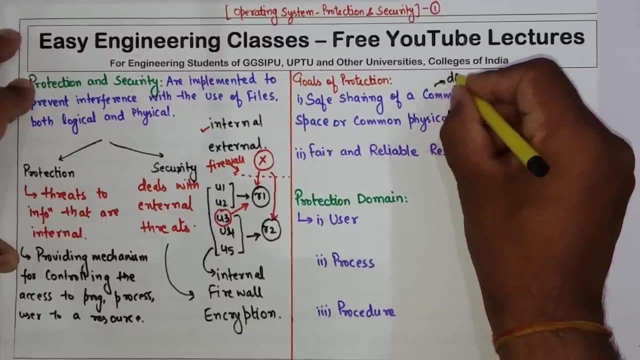 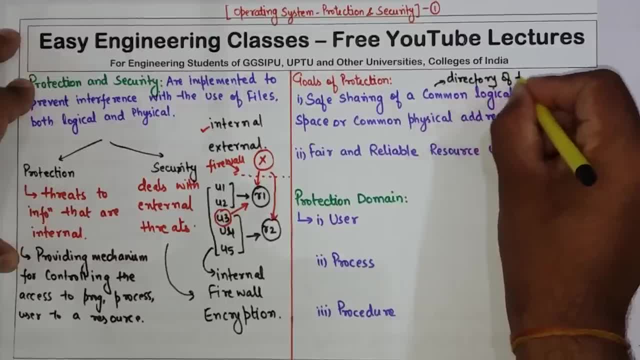 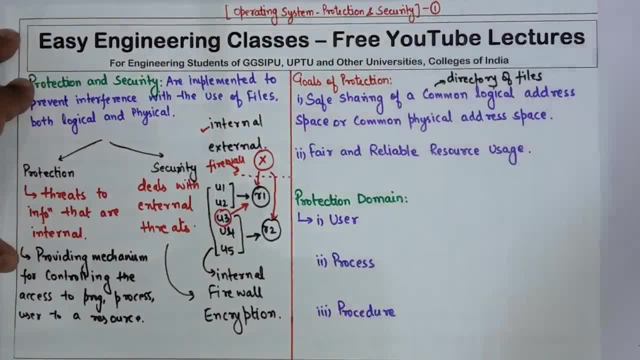 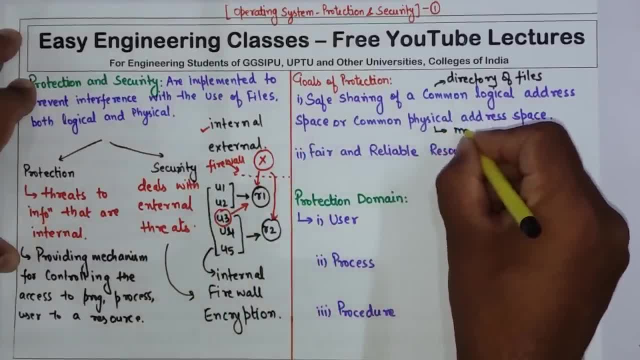 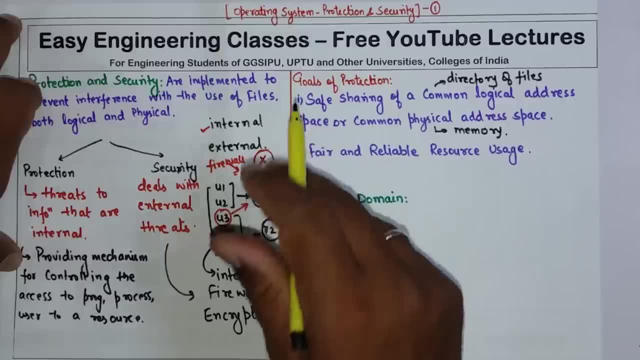 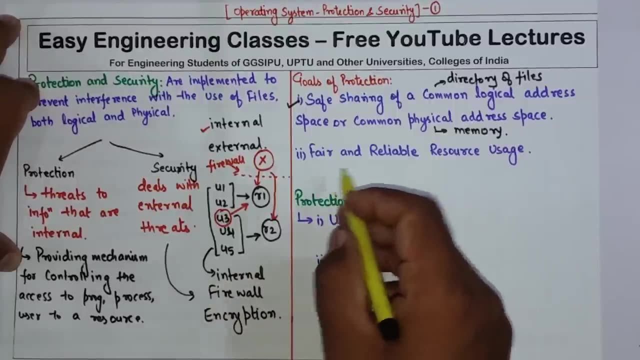 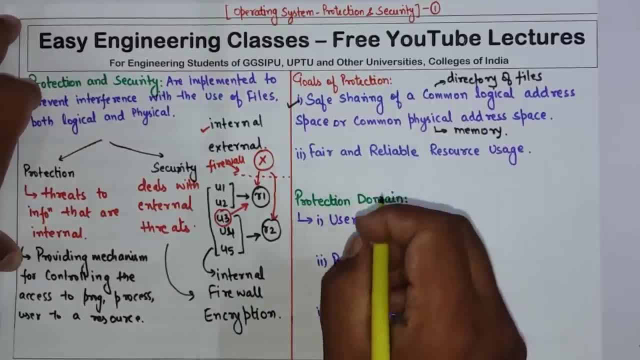 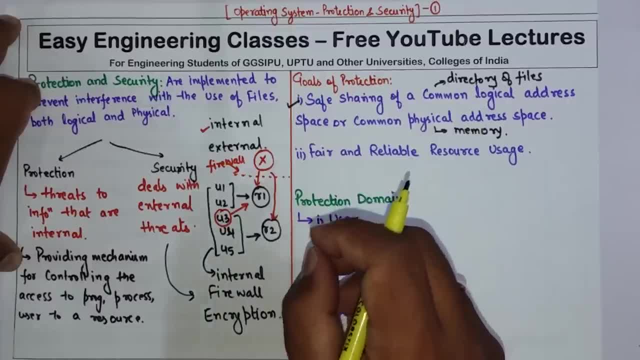 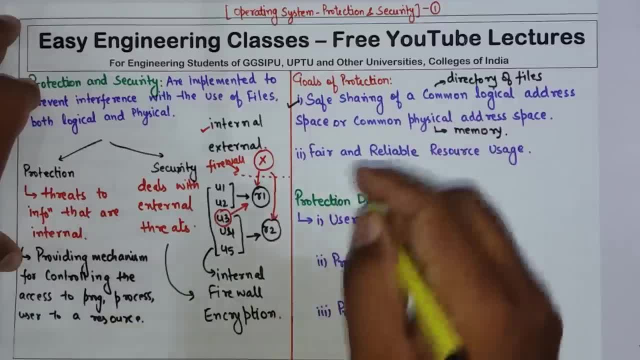 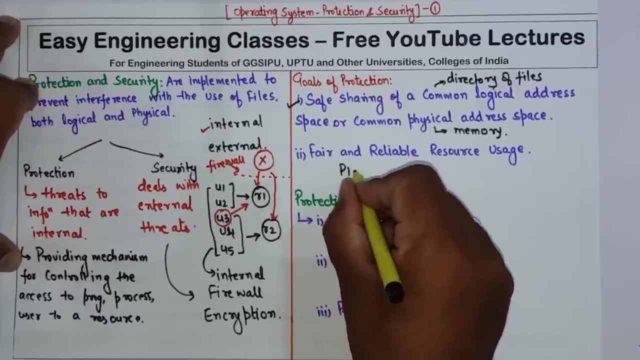 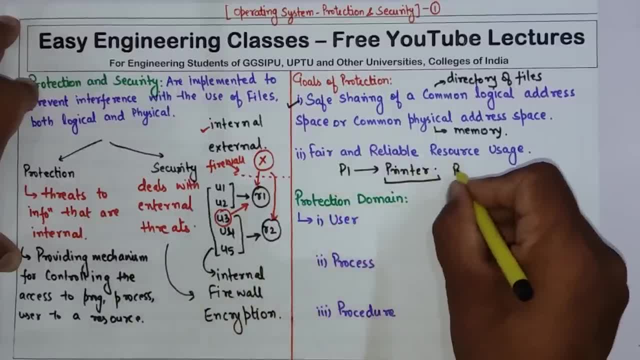 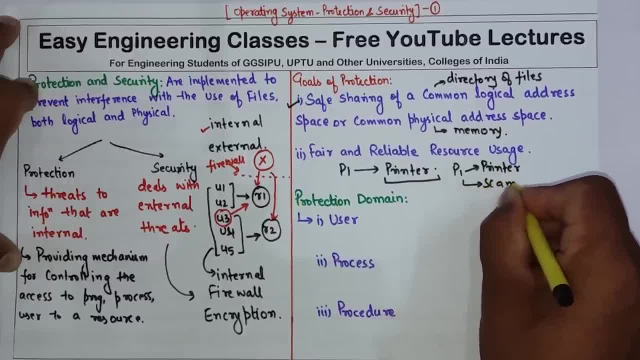 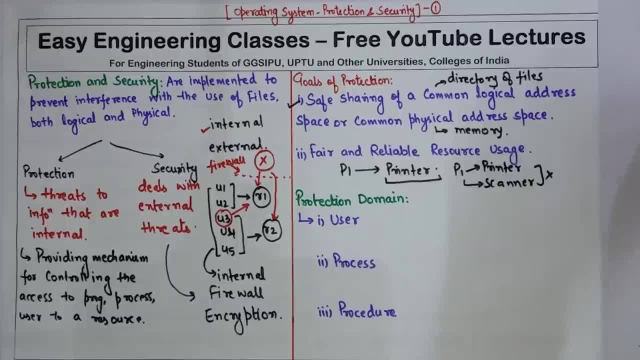 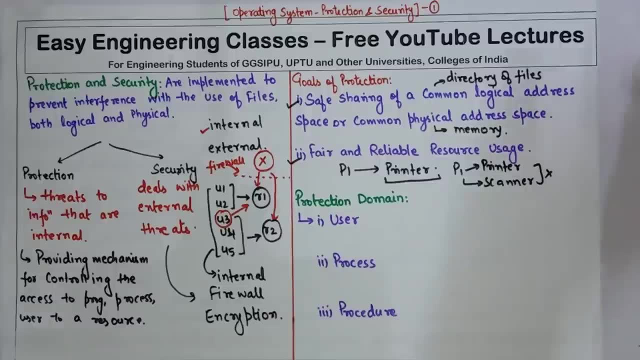 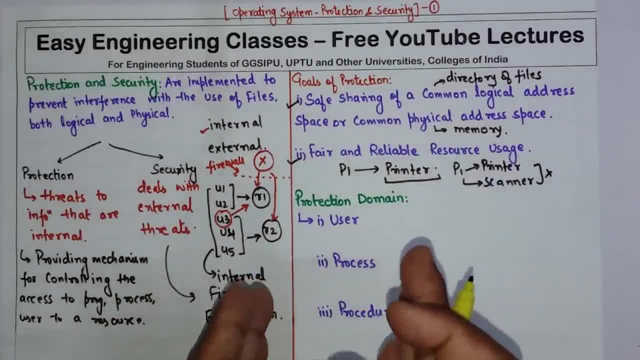 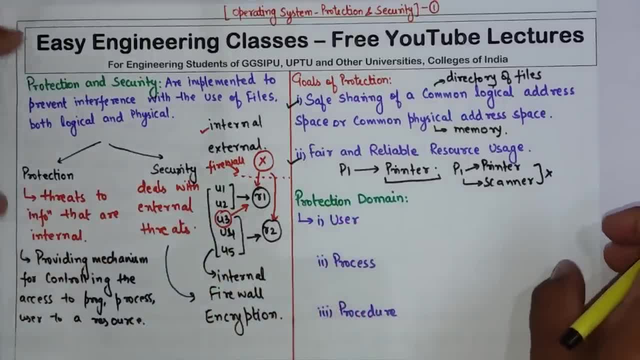 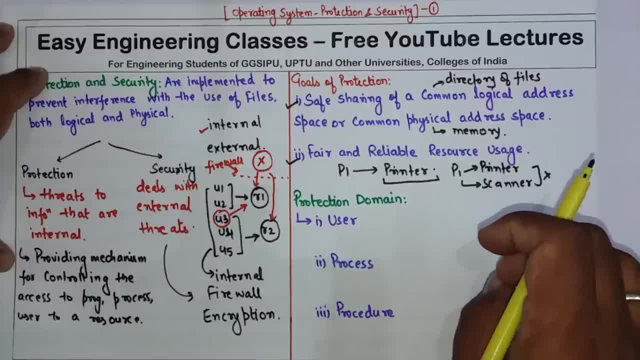 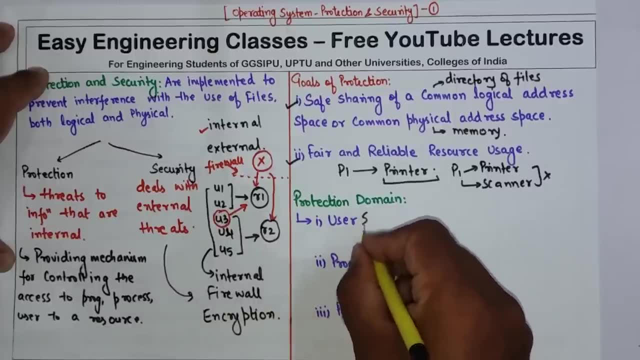 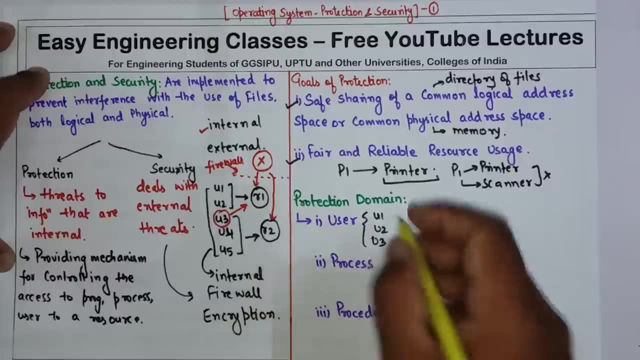 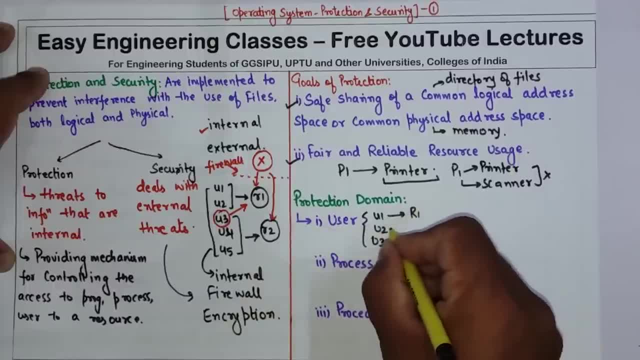 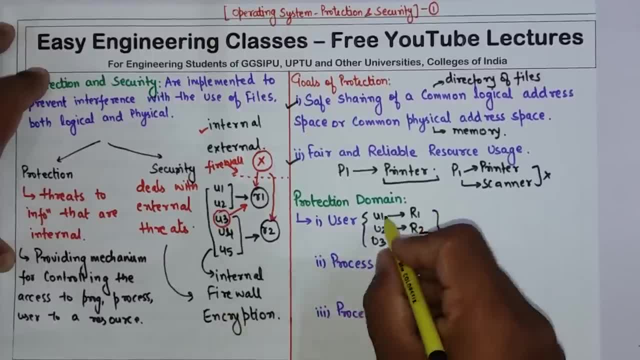 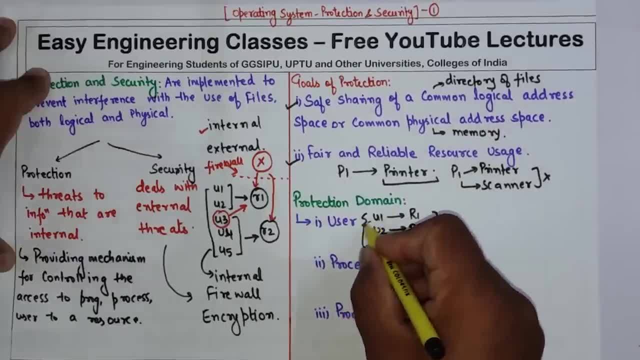 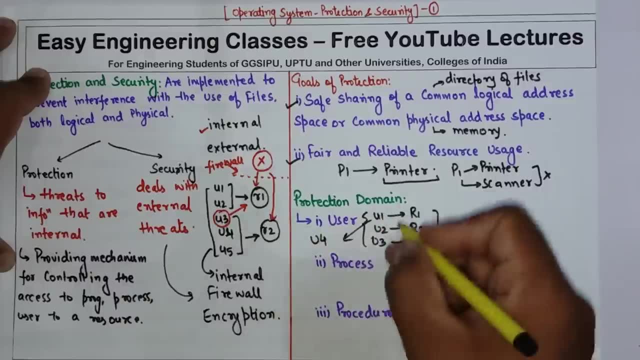 so if the user is changed- suppose user u1 is now changed to user u4. so what we are doing is we are switching the domain from u1 to u4, so domain switching may occur. now a process can also be a domain, similarly, as we have used the user id as the identifier in this case. 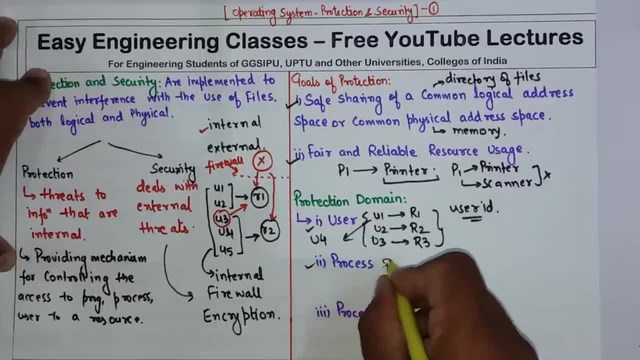 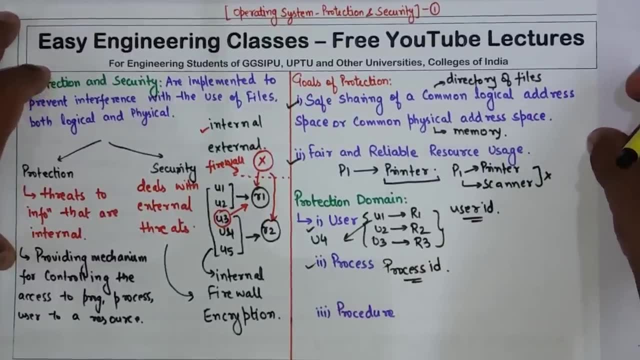 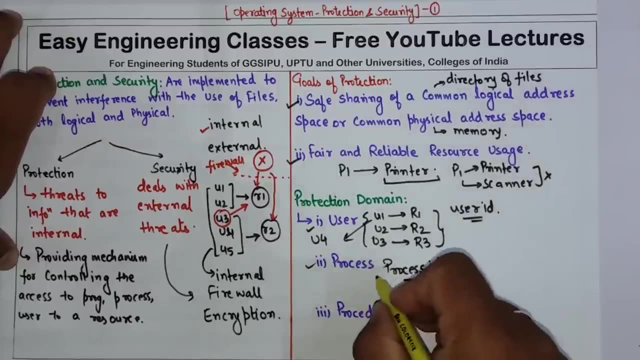 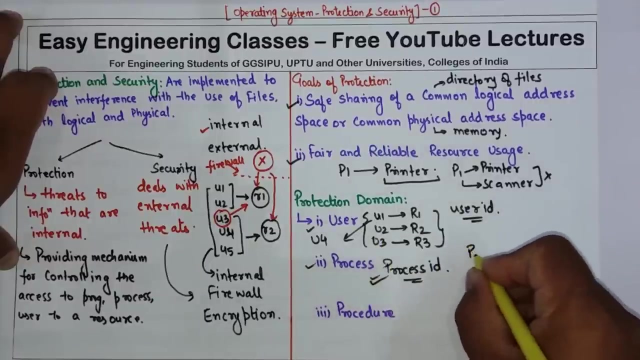 in process, the process id is used as the identifier and each process is like a domain. now, the resources that can be accessed depends on the identity of the process, which is done with the help of process id. so in this case, now, the process ids are used to define the domain. 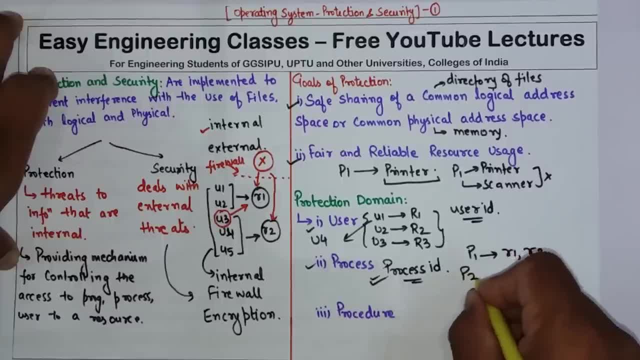 for example, process p1 can access r1- r2, so in this case the process id can be used to define the domain. so in this case the process id can access r1- r2. Similarly, process P2 can access R3, R4.. 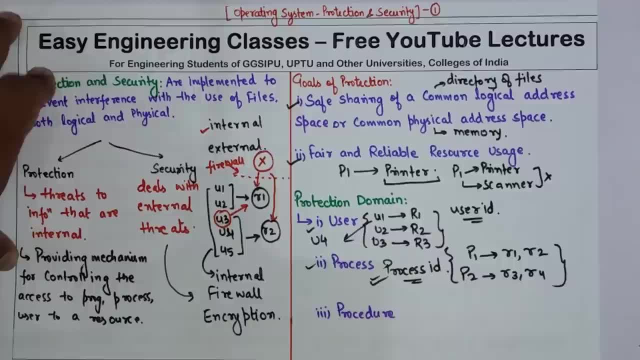 So in this way, the domain of the processes are defined. In the same manner, procedure can also be used as the domain. Now, in this case, the set of objects that can be accessed corresponds to the local variables defined within that procedure. 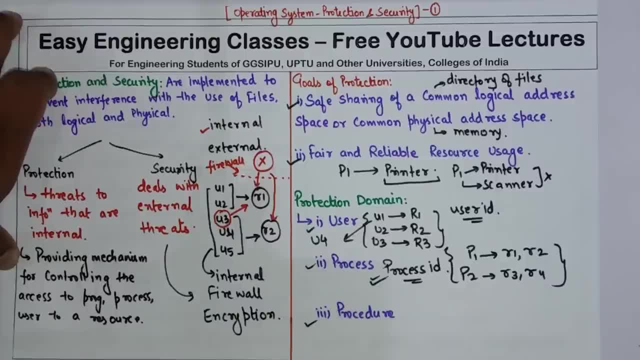 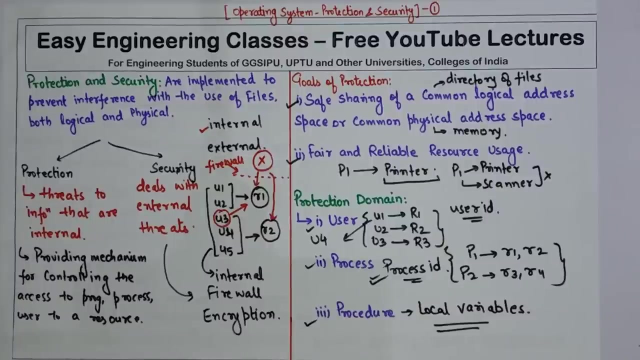 So now the variables that are defined in the procedures are used to control the access of the resource. So in this you can write: local variables are used to define the domain of the resource that can be used with this procedure. So this is a brief about the protection and security. 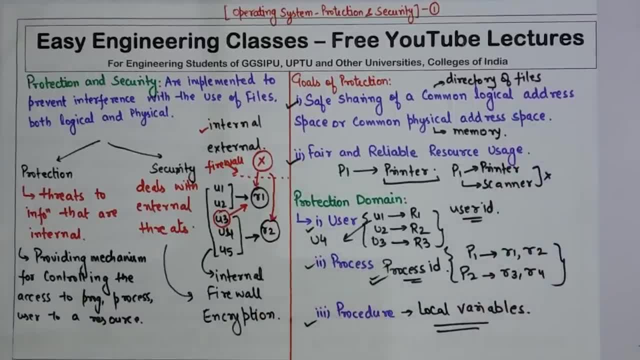 Goals of protection and the protection domain. In the next video, we are going to see the access matrix, which is the most important point of this topic- protection and security- So keep tuned to my YouTube channel. Thank you for watching the video. Please subscribe to my YouTube channel for more such tutorials. Thank you. 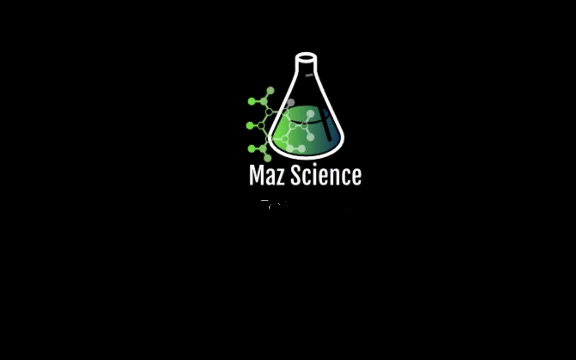 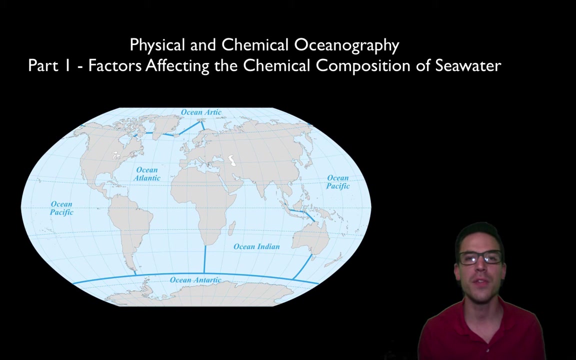 Hi guys, and welcome to our first video in unit 7 on physical and chemical oceanography. In this video, we're going to be taking a look at factors affecting the chemical composition of seawater. Now, oceans cover about 70% of the Earth's surface and, as you might be aware of already, not all of 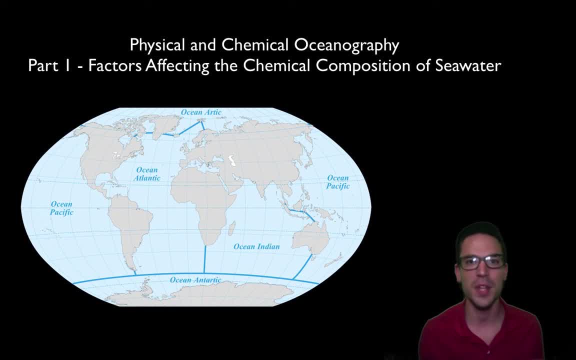 the oceans is 100% water. There are going to be different things dissolved in that water and those things are important because that's going to ultimately affect the different kinds of life that we find living in the oceans, as well as their distribution. So in this video we have 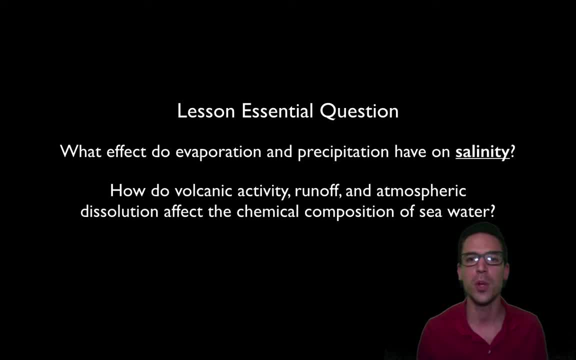 two essential questions. Our first question is going to be: what effect do evaporation and precipitation have on salinity- and we'll go over what salinity is and what salts are here in a second- and also taking a look at how volcanic activity runoff and atmospheric dissolution. 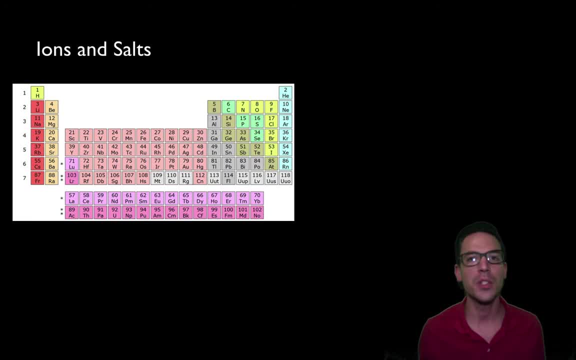 affect the chemical composition of seawater. So before we can talk about salinity, it's important for us to have an understanding about what is meant by the term salt. Now, you might be familiar with table salt already, or sodium chloride, but that's not the only salt that. 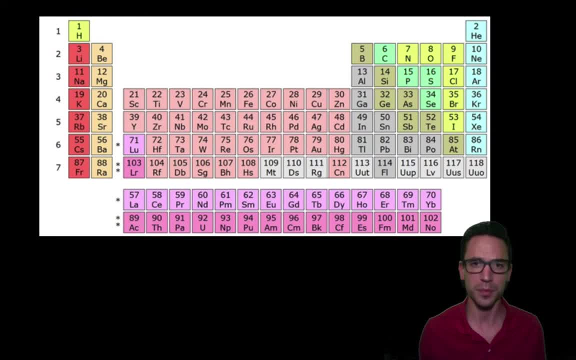 exists. So just looking at this periodic table of elements, you don't have to memorize the whole thing. but just something I wanted to touch on was the concept that atoms and molecules have a tendency to either give up or gain electrons, and that's going to give them charge. So we're 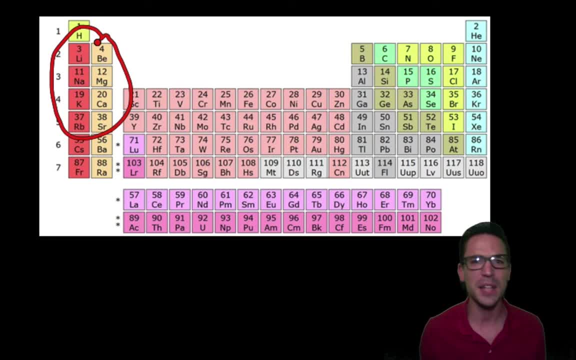 to just look at the atoms that we find on the left side of this chart. These guys typically have a tendency to give up or lose electrons and because of that, they're gonna have more of a tendency to gain electrons, which is going to give them more of a negative charge and any time.